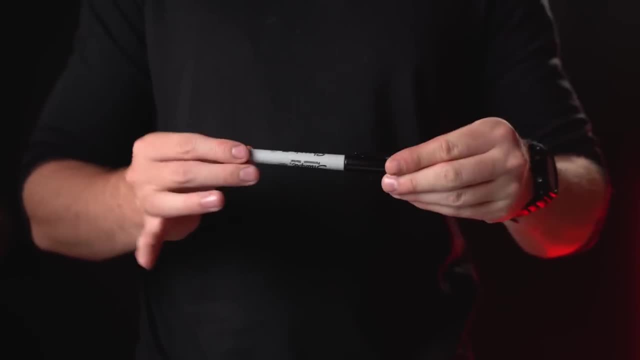 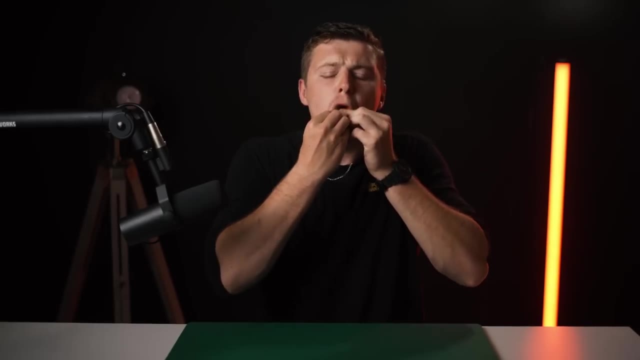 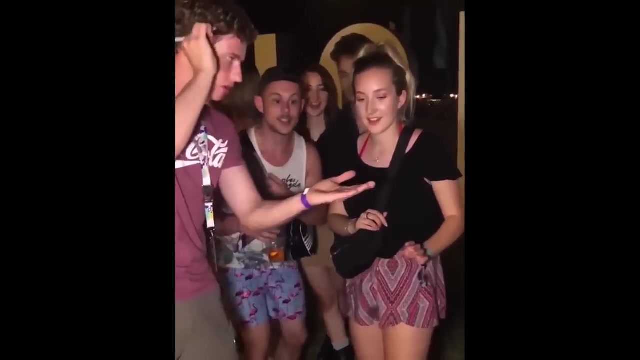 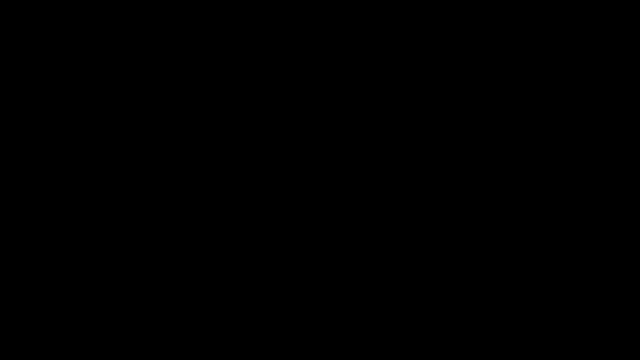 Watch the pen as it visually vanishes. The coin instantly disappears. I can make the pen go up my nose And I'm even going to teach you this hilarious party trick where you make a pen vanish. Hey guys, welcome back to the channel. In this video I'm going to be teaching you five. 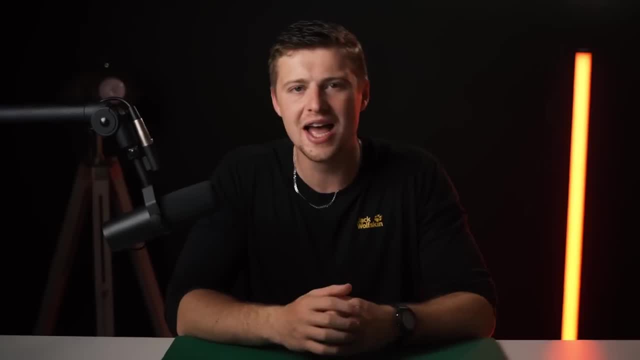 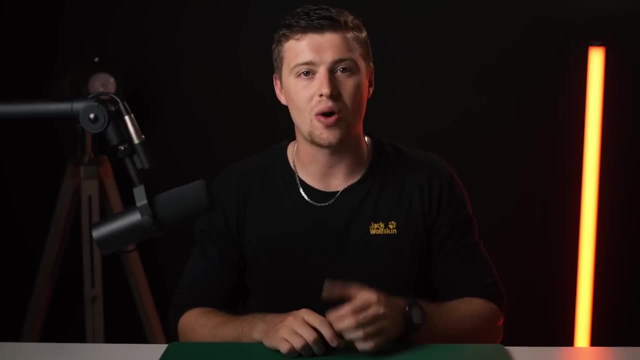 super fun and super visual pen tricks that anyone can do. Now, these aren't like whole magic performances. these are just little gags that you can pull off at school or in the office, so I hope you enjoy learning them. So we've got a pen here. 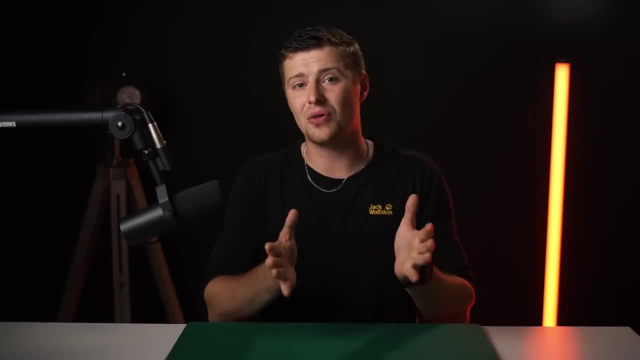 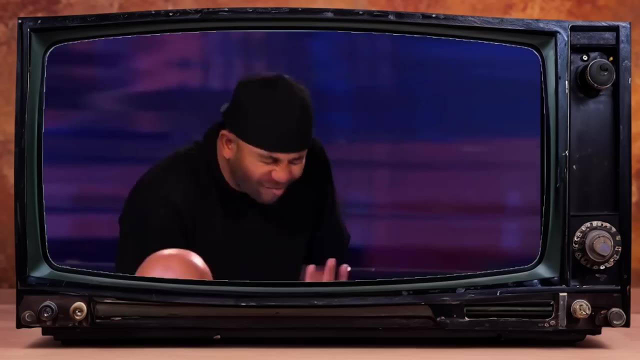 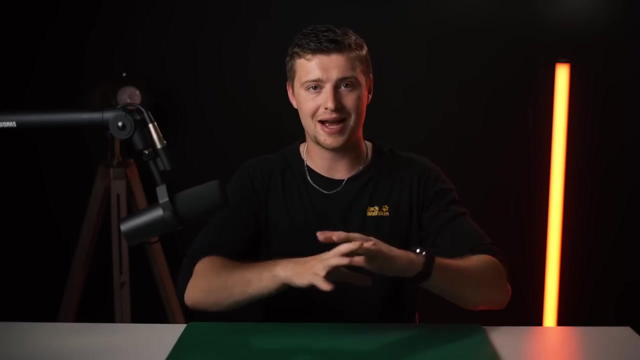 And we can make it go up my nose and out my mouth And, believe it or not, this effect has actually been done on America's Got Talent, as you can see here. So it really is good enough to impress thousands of people in a massive stage and people close up as well. 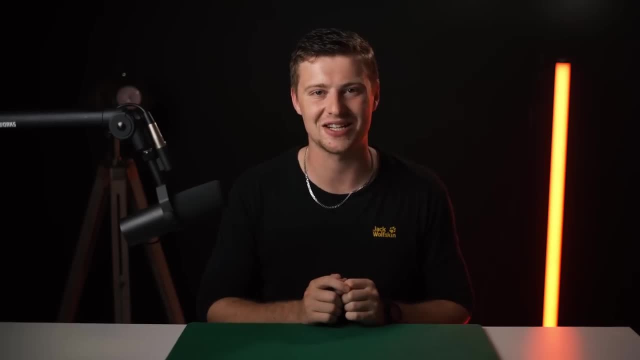 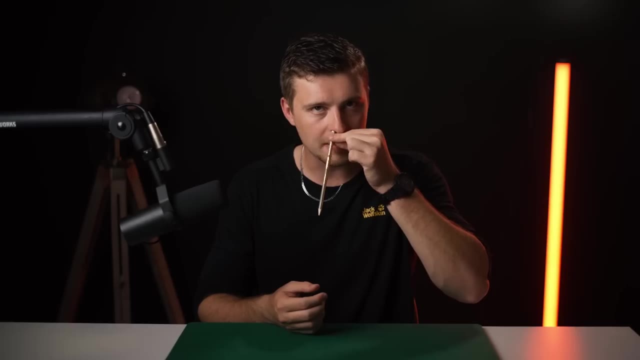 So definitely learn this amazing trick. So the way this works is very simple. Simply take a pen or pencil and hold it at the top with your two fingers here and then place it on your nostril. Then all that's going to happen is these fingers together are going to slide up the pen and it 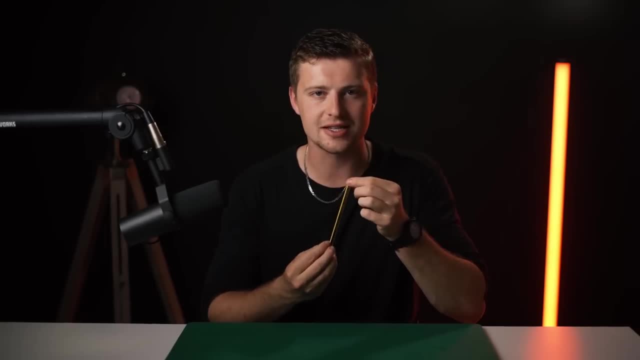 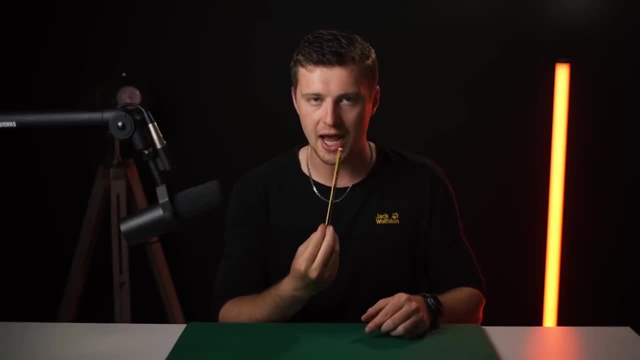 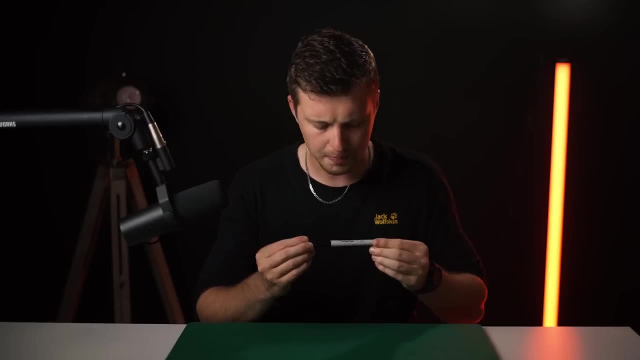 And then you've got the pen going up your nose And then you simply bring it down into your mouth and put it out like that. So it's a very quick, simple trick. you can do with any pen or pencil Very quickly. if you want to become a more interesting person, then definitely subscribe. 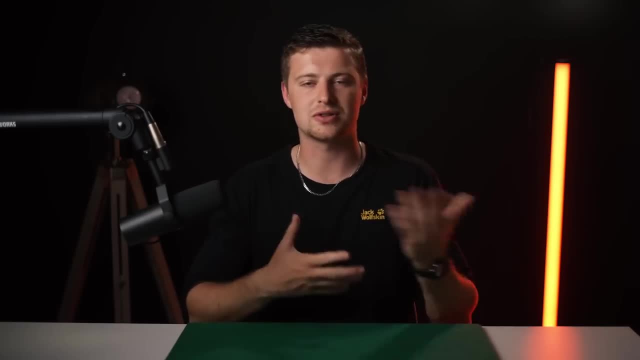 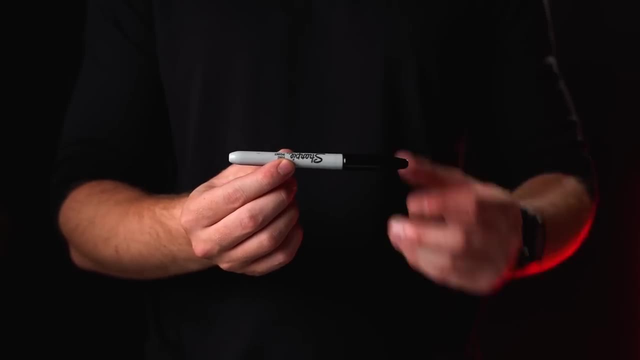 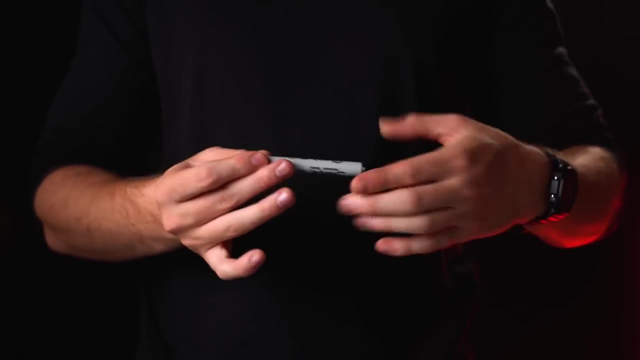 to this channel as I teach loads of amazing effects like this That will just help you become more interesting and more well-rounded. Watch the pen as it visually vanishes. Watch the pen as it visually vanishes. So in order to do this vanish, what you need to do is hold. take a normal sharpie or any size pen. 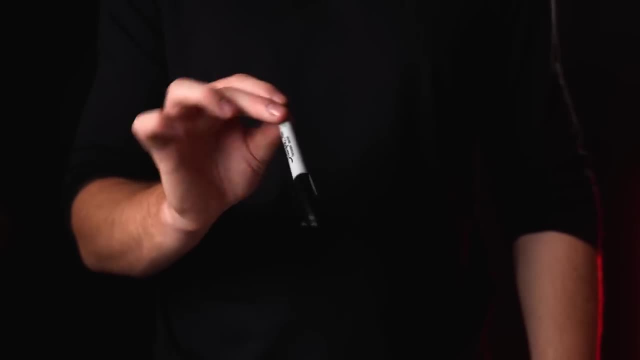 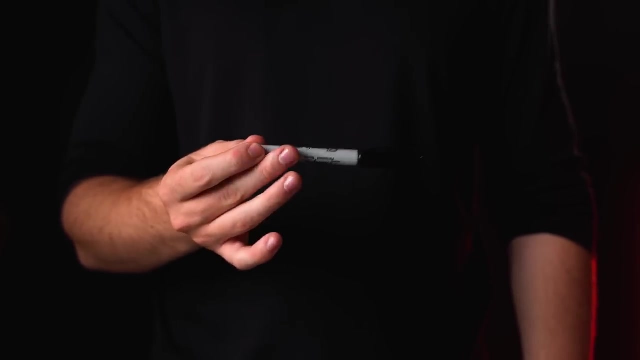 and hold it between your first finger, your middle finger and thumb, just like this. Then you need to extend your middle finger and pull back on the pen. Just practice doing this over and over again and you want to get it to the point where it's quick. 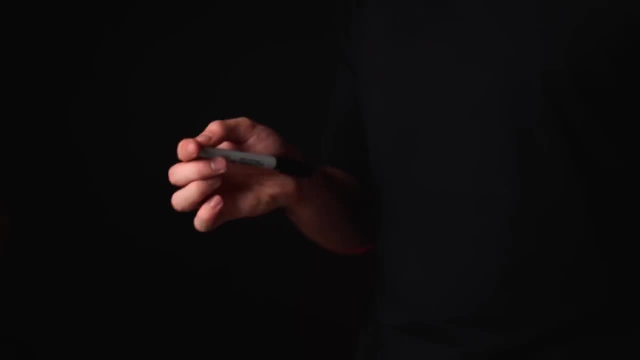 So once you can pull back the pen confidently, the pen goes back here. Use your thumb to then push the pen down. Use your thumb to then push the pen down. Use your thumb to then push the pen down. Use your thumb to then push the pen back out. 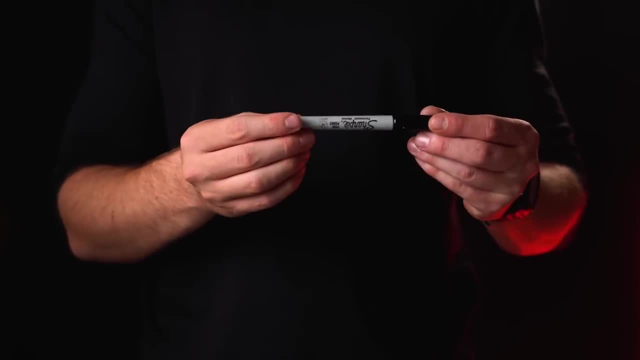 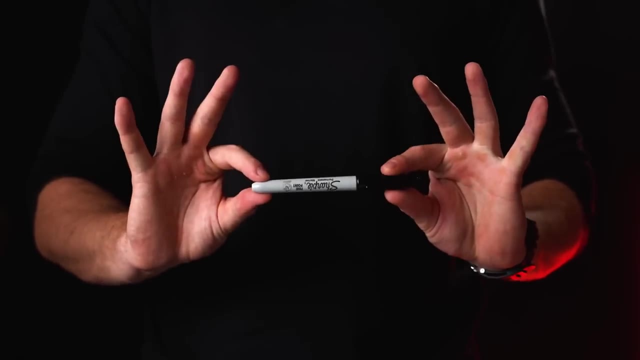 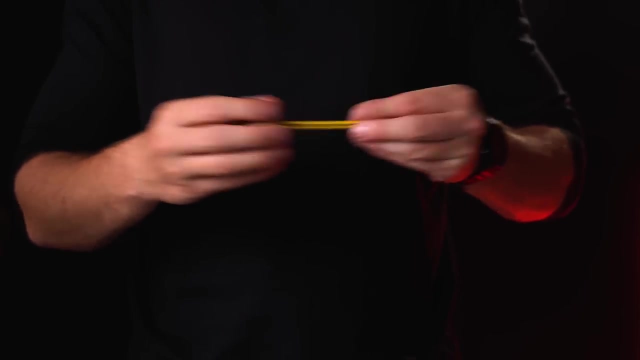 Practice doing this, move over and over, and once you're comfortable with it, you're just going to do it under the cover of your other hand and the pen will appear to vanish. So the magician has a pencil, He passes the pencil in between his hand and the pencil gets really small. 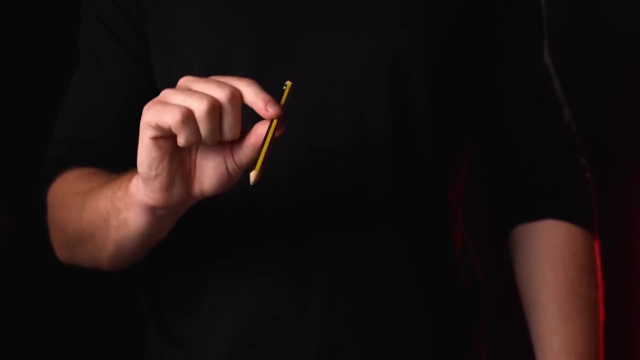 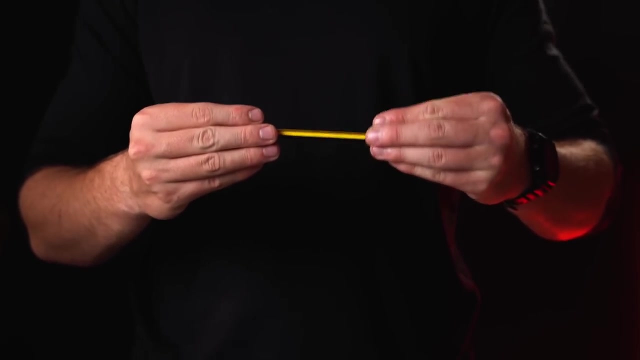 And then the pencil grows back to its full size. So this is just a very quick illusion. you can do with any pen or pencil. So this is just a very quick illusion. you can do with any pen or pencil. Hold the pen or pencil between your fingers, but make sure all your fingers are together like this. 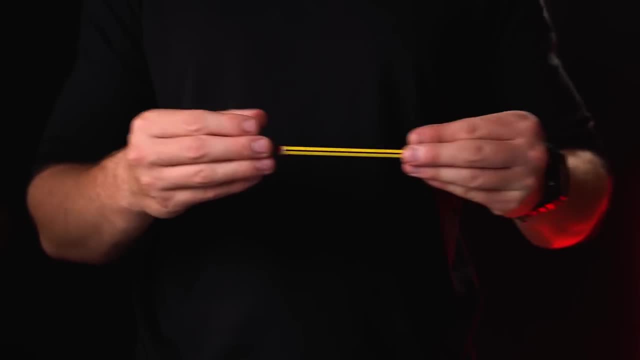 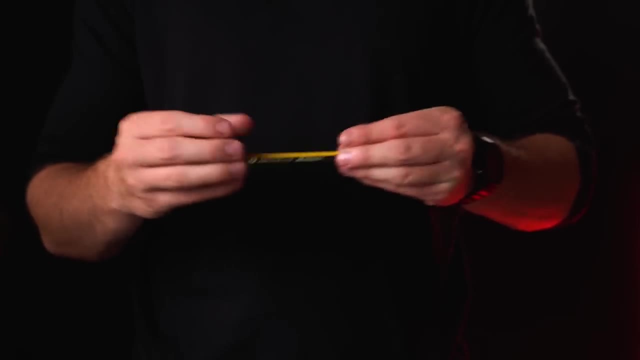 Then you want to pass the pen in between your hands and because half the pencils at any given point has been covered up, when you do it quickly, it looks like the pencil is really small. So practice this in front of the mirror. just give it a go and you'll be able to. 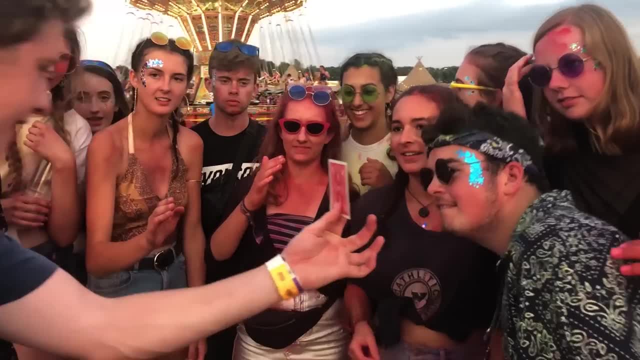 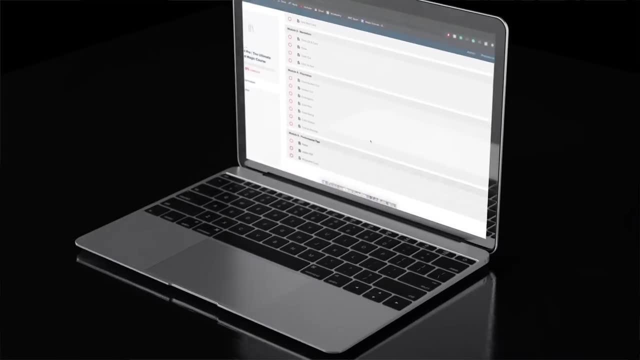 learn this really cool illusion in a few seconds. Now, if you want to become a real wizard, then consider checking out my course, Card Magic. It's the most popular card magic course in the world, with over 10 000 students, and it just teaches you tricks and slights that are way too good to reveal on YouTube. 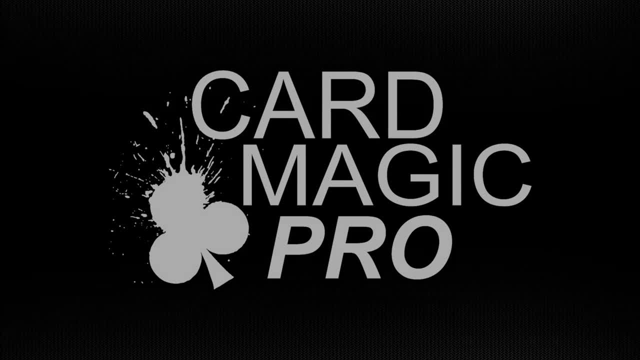 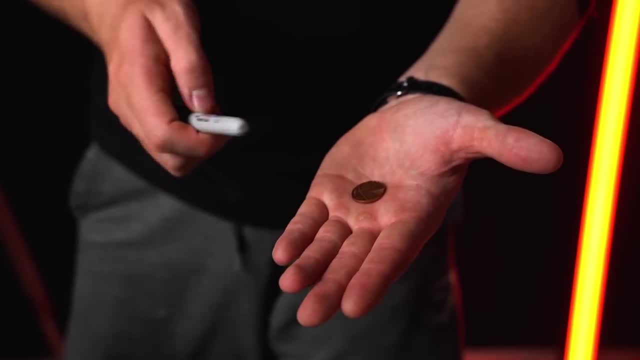 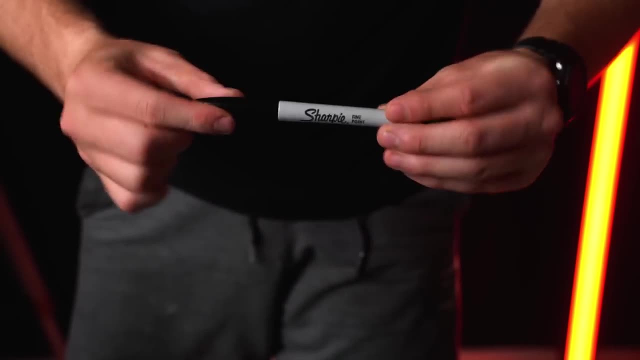 So I've left a link down in the description to where you can check it out. The magician has a coin and a pen and he says he's going to make the coin vanish by tapping it. The coin completely vanishes. So in order to do this illusion, just take a pencil. 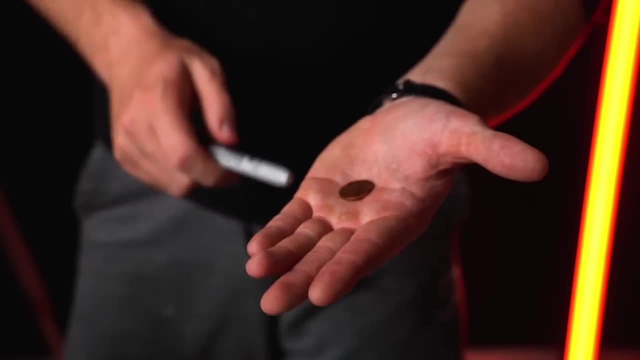 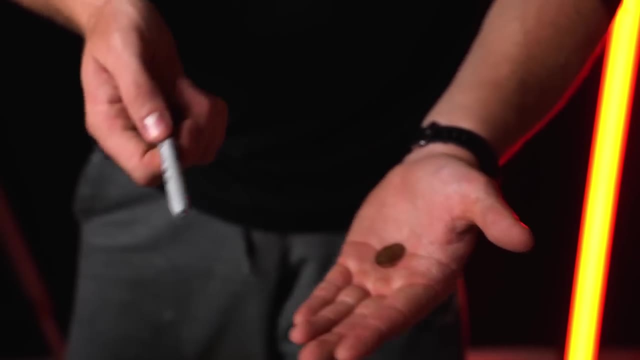 Any coin at any pen and you're just going to tap the coin three times. So you tap it once, you tap it twice and then, on the third tap, you need to make these fingers slightly looser and just open them up slightly, and all that's going to happen is the coin is. 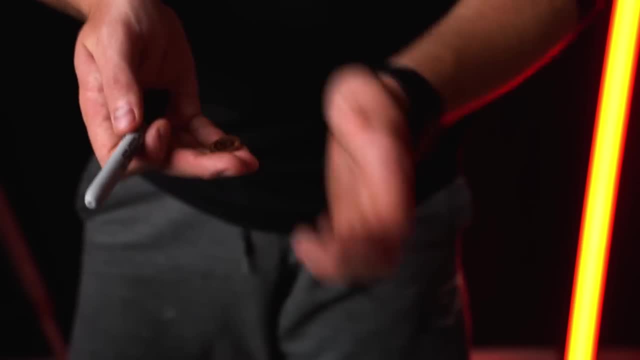 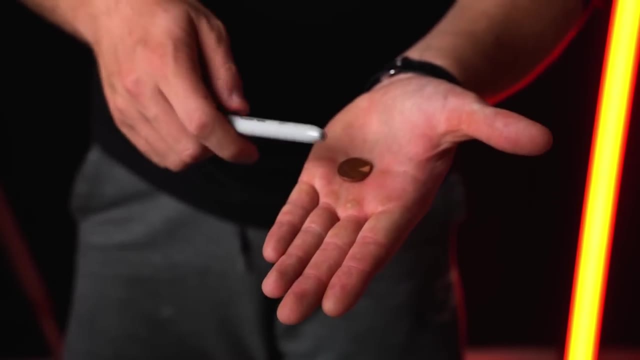 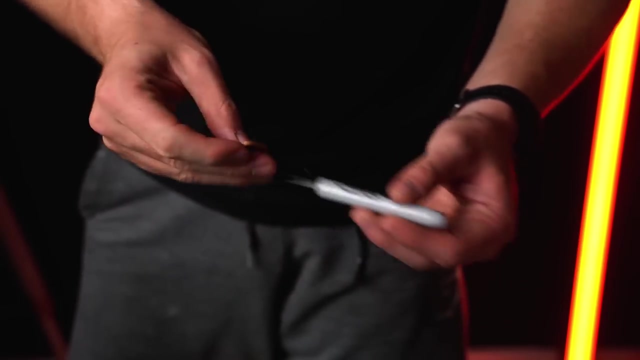 going to be chucked from this hand into these fingers here. So you're just chucking it in there like that, but at speed. it creates the very convincing illusion that the coin is visually gone. So just practice doing this over and over again And you'll be able to catch the coin in this hand.